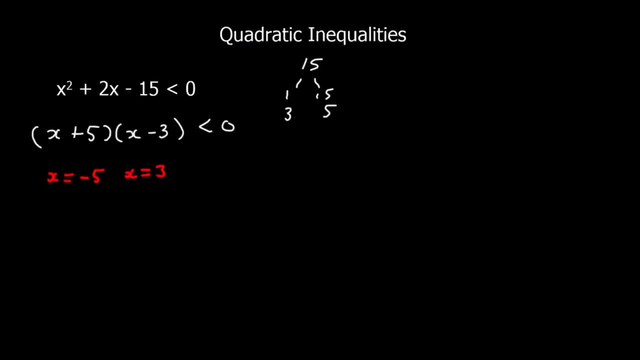 So x would be minus three. take away three, So x would be minus three. take away three, So x would be minus five and x would be three. So that's the points where it equals zero. So if I was going to draw this on a graph, it will cross at minus five and it. 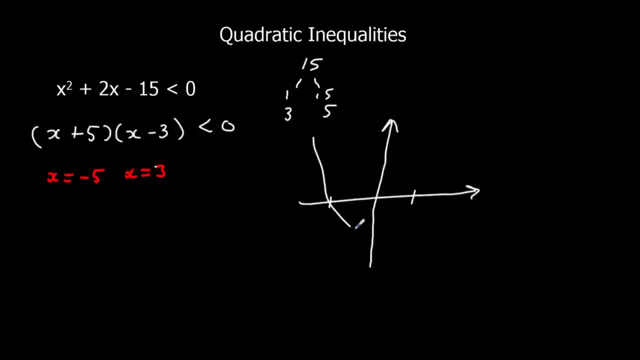 will cross at three. So it's a quadratic graph. So I look at that at minus five and at three. Now we want where it's less than three. So we're going to take away three, take away three. So if I was going to draw this on a graph, it will cross at minus five and at three. 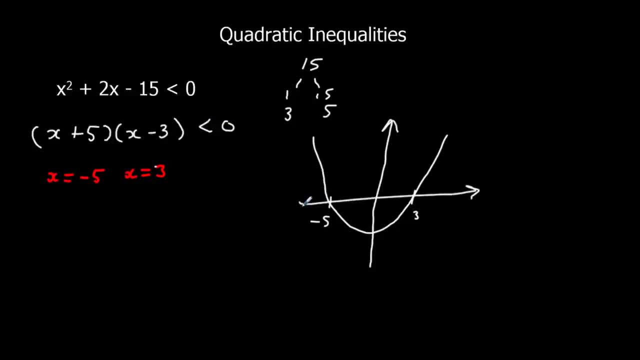 Now we want where it's less than zero, where this graph is below zero. So zero is here. this is zero. that's the zero line, that's ground level. So we want to know where it's below ground level. So it's this bit of the graph. So what are the x values for this bit? 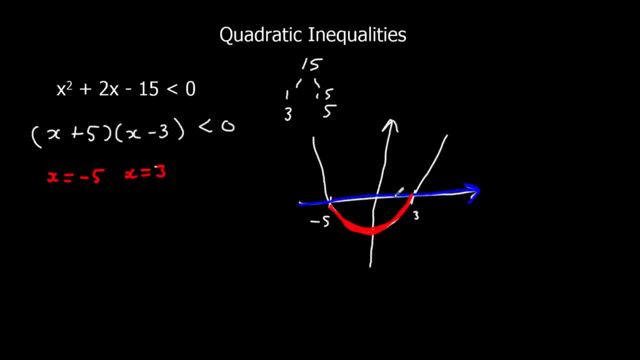 of the graph. It's in between minus five and three. X has got to be bigger than minus five, but less than three. We knew from factorising that these two values were going to be involved in the answer. We just had to find out where. So we want below zero, where it's less than. 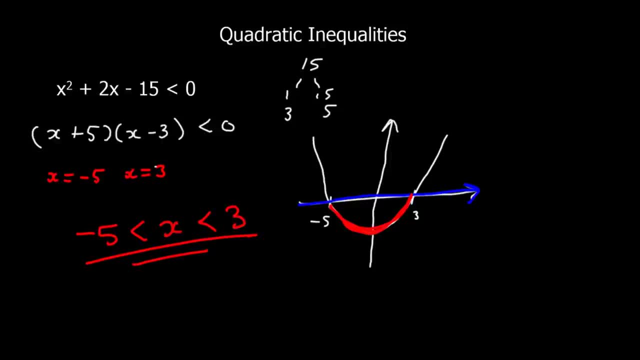 zero, that's in between these two values. Okay, this example, it's got a bigger or equal to zero sign, But the first step's the same. So we're going to go two brackets, Factors of 12, one times 12, two sixes, or three fours. 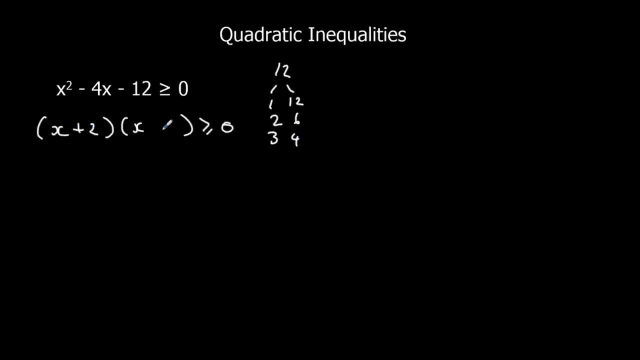 I want minus four, So I'm going to do plus two. take away six. So if it was equal to zero, or it is equal to zero at minus two and at six, So that's where it's equal to zero. 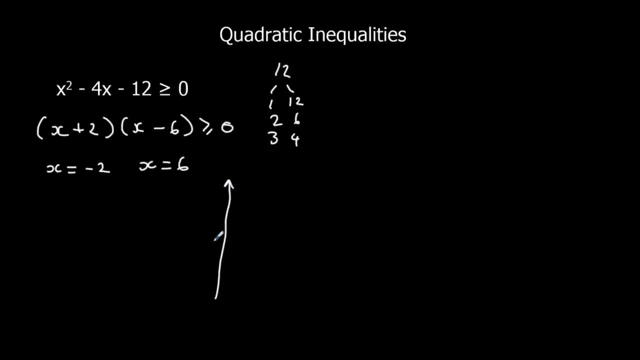 But we need to know it's bigger or equal to zero. So it crosses at minus two and six. So parabola, it's a U shape And we want it's bigger or equal to zero. So bigger means above ground, above the ground level. So it's this bit of. 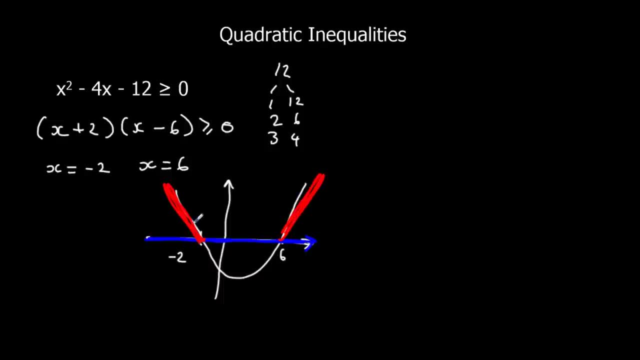 the graph here and this bit of the graph up here. So what's x for these? Well, it's going to be less than minus two Or equal to minus two, because it can be minus two, Or it's going to be bigger or equal to six. So it's the two upper bits When it's bigger than zero. 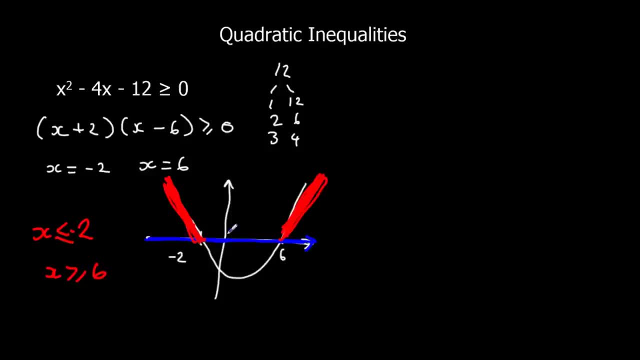 it's the two upper bits of the graph. When it's less than zero, it's the bit underneath the lower bits of the graph. So they are our answers. Okay, so let's go through what each of the signs means in terms of the answers. 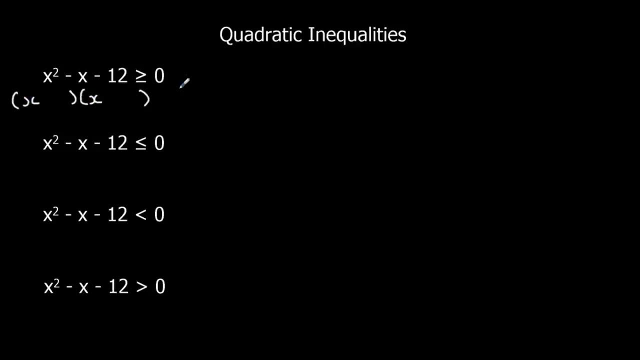 All of these are going to factorize Factors of 12, 1 and 12, 2, and 6,, 3 and 4.. We need minus one, so it's plus three minus four. So all of these equal zero at minus three and at four. 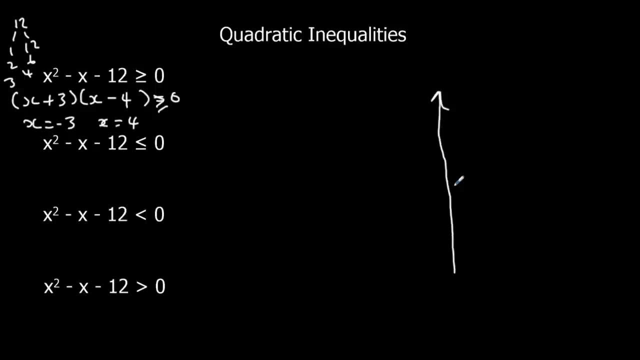 So the graph is the same for all of them. It's going to go through minus three and it's going to go through four. So this is what the graph looks like for all of these questions. We just need to know what part is bigger or equal to zero for the first one. So bigger or equal to zero? 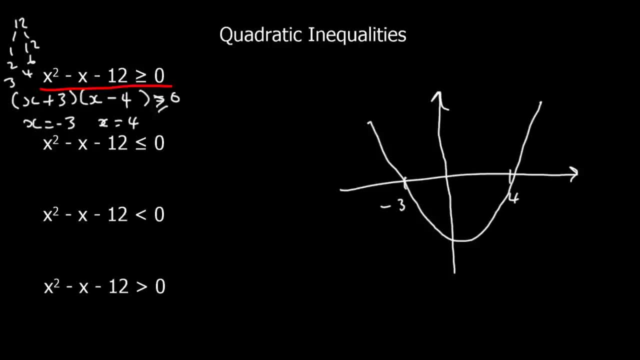 For this one than zero. so that means above the ground. this is the ground level. this is zero. where's the graph bigger? well, it's up here and up here. so it can be for x. what can x be? it's going to be less or equal, because it can equal it to minus three, and it's going to be. 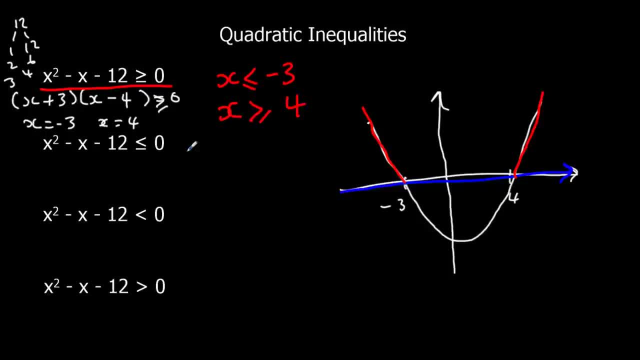 bigger or equal to four. okay, for this second one, we need to know it's less than or equal to zero. where is it less than zero? underground down here? this is where it's less than zero. so for, in terms of x values, it's between minus three and four. 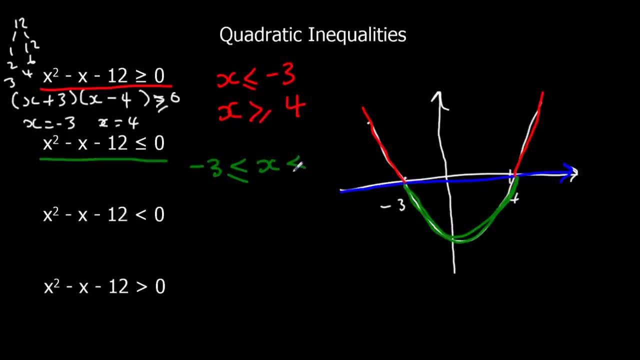 it's bigger or equal to minus three and less than or equal to four. okay, this one says less than. so we're talking about the same part of the graph as less than or equal to, but it just can't equal those critical values. so it's just exactly the same, but it can't equal. 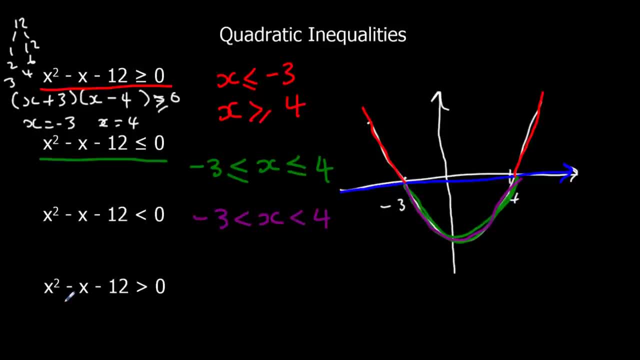 those critical values and for this one it's the same as this one. it's the top parts of the graph, so it's going to be less than minus three and bigger than four. it just can't equal them like it can here. okay, see if you can give these two. 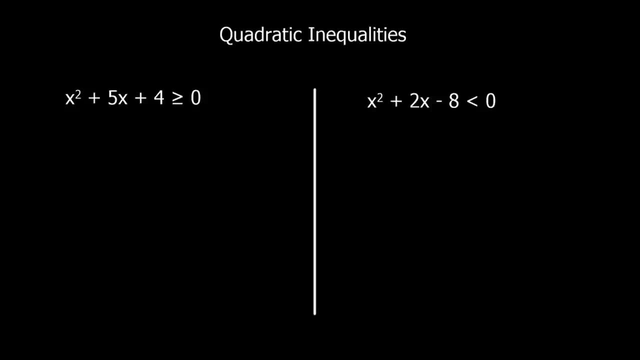 questions here. okay, first step, we're going to factorize. so x, x factors are four, four and one, or two and two. it's going to be four and one. so it's going to equal zero at minus one and it's going to equal zero minus four. so in terms of the graph, it's going to go through. 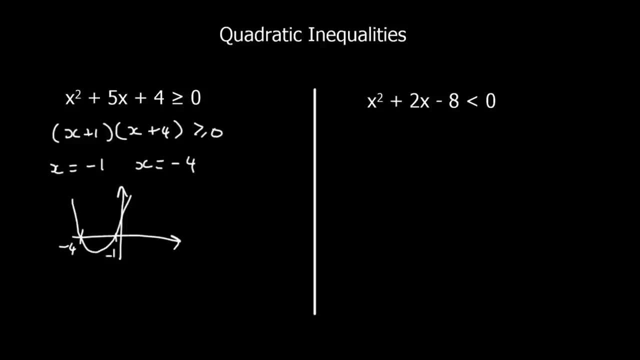 minus four and minus one. so we want where it's bigger or equal to zero. it's the ground level is worth equal to zero. where is it bigger than above the ground? so x is going to be less than minus four and x is going to be bigger than minus one. 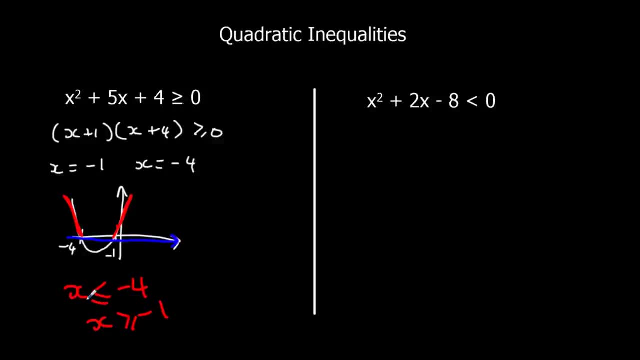 or or equal to sorry, it's an- or equal to question. so it can equal minus four and it can equal minus one. okay, here we're going to two brackets again. factors are eight, one times eight, two fours. we want plus two, so it's gonna be plus four. take two: it equals zero at minus four and two. 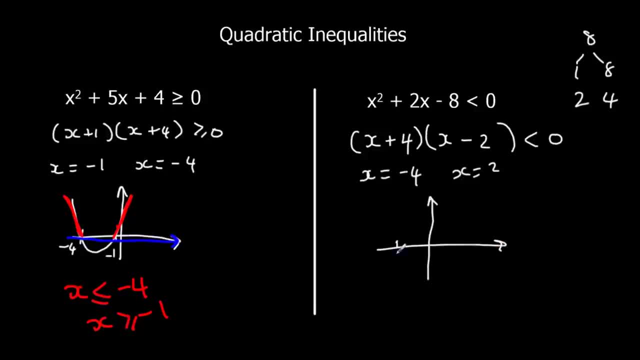 so equal zero at minus four and two. we have four plus two. we take two. it's going to be zero at minus four and two. We want to know where it's less than 0. So where it's underground, what are the x values when it's underground?